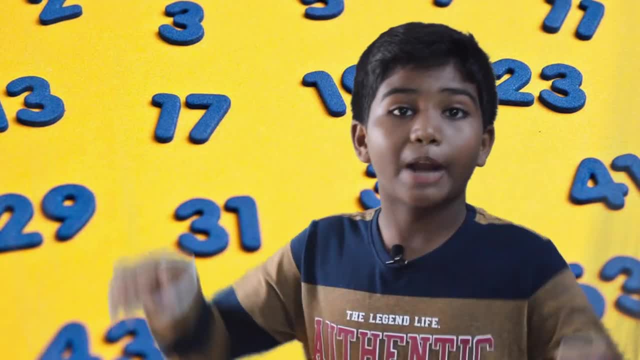 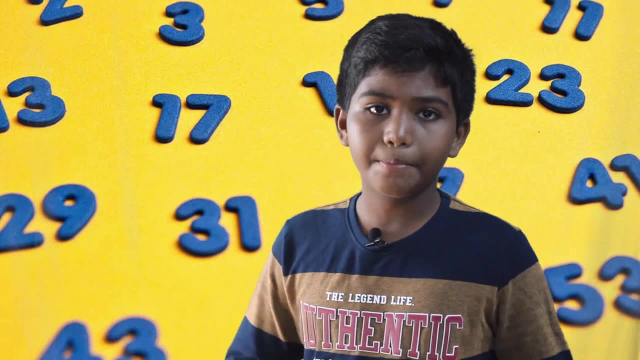 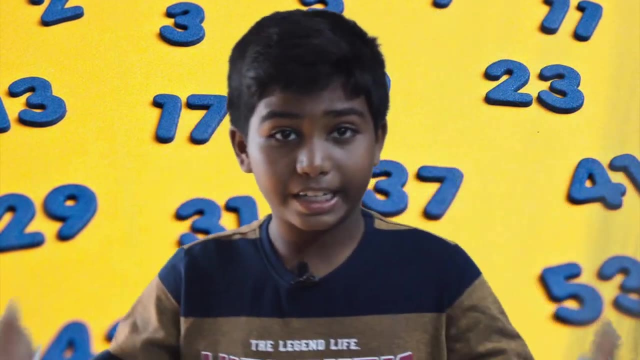 We have an infinite number of prime numbers, just that they will occur less frequently in the number series as the numbers get bigger. So throughout the world there are many prime numbers Throughout our number series, starting from 1 and going on infinitely. we have infinite prime numbers sprinkled in the series. 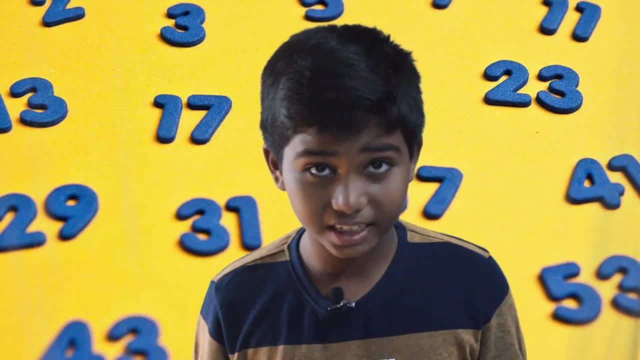 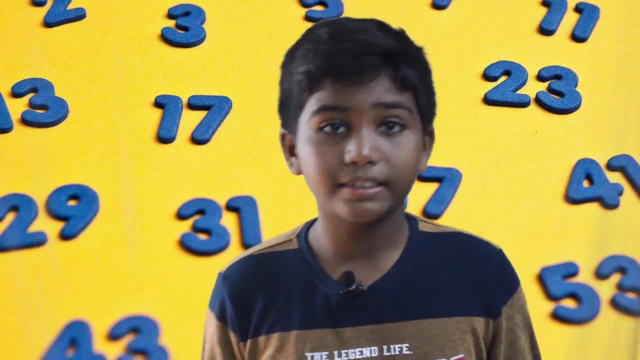 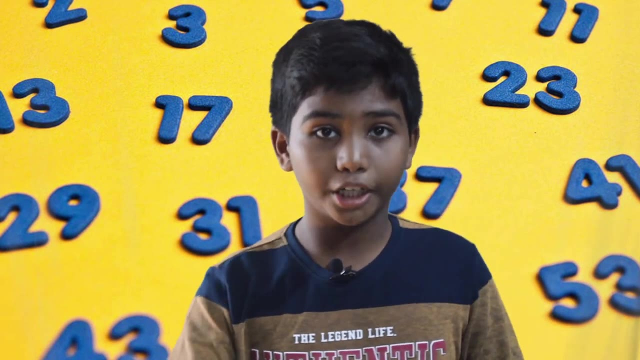 And, interestingly, all of the numbers in the series can be produced simply by using prime numbers. For example, 20 can be written as 5 into 2, into 2.. 100 can be written as 5 into 5 into 2, into 2, and so on. 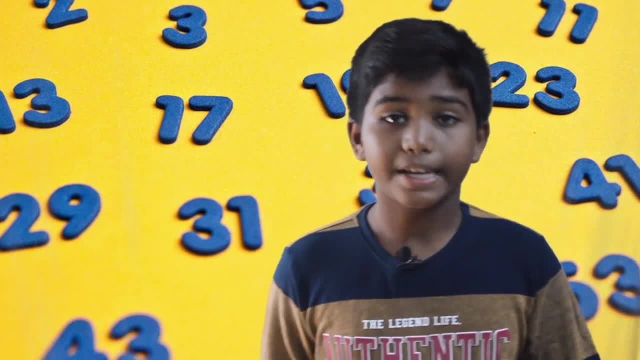 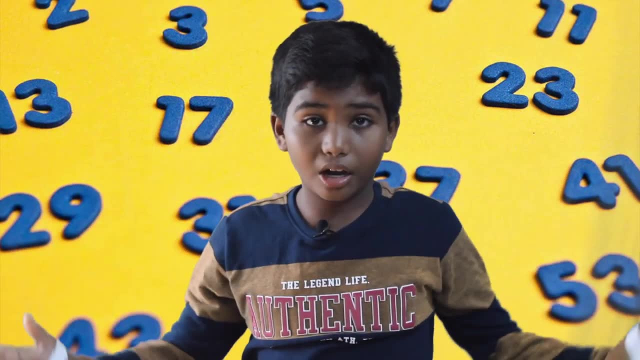 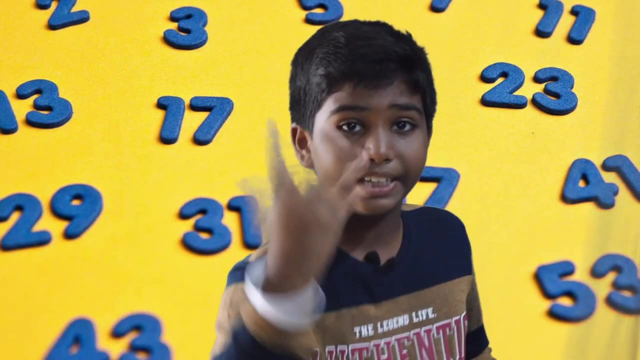 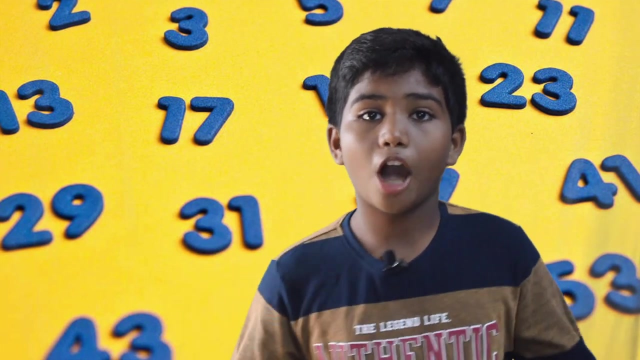 In this context, prime numbers can be referred as basic level numbers. It is because we can pick any number and write it in terms of multiples of other numbers. When no more factoring can be done, we are left with primes. Also, in this sense, primes can be called as building blocks too. 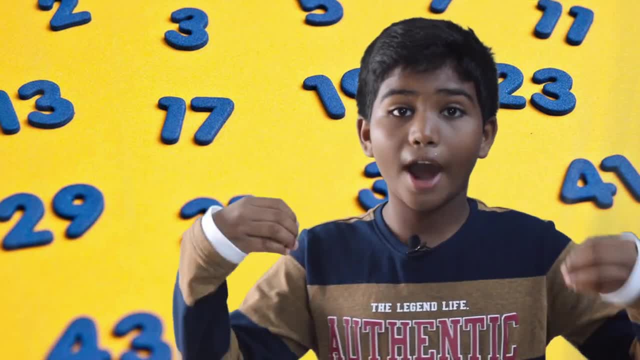 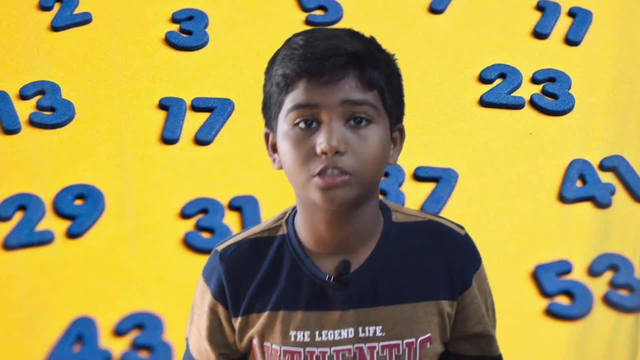 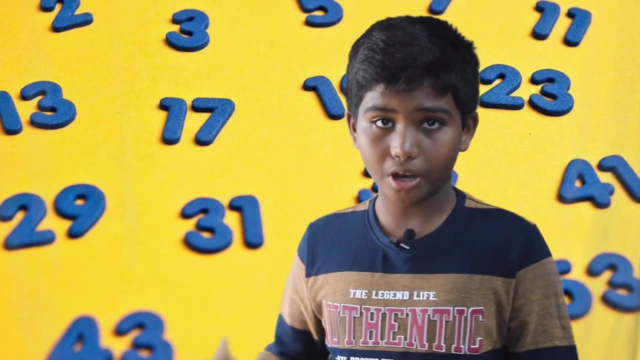 This property of factorization is what makes Prime numbers interesting and hence useful. So we can multiply a heap of prime numbers to find a really larger number. However, when you are given with a very large number, factoring it back into prime numbers is not easy peasy. 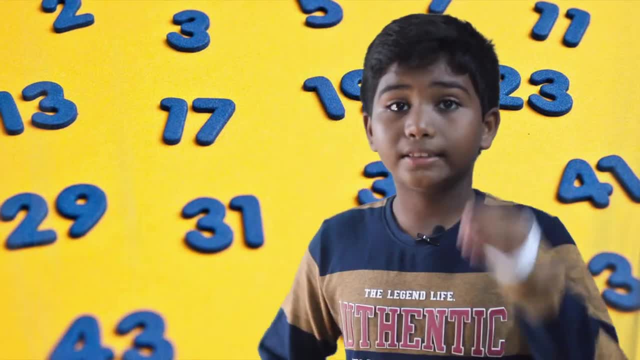 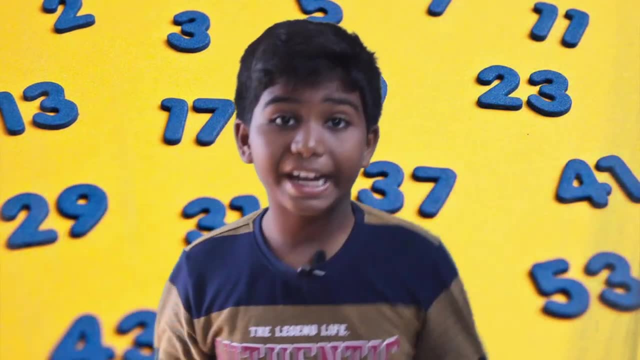 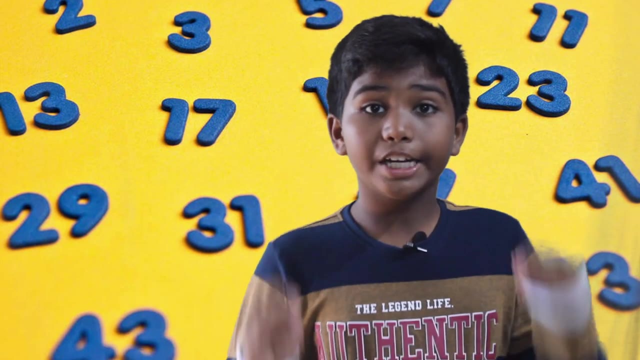 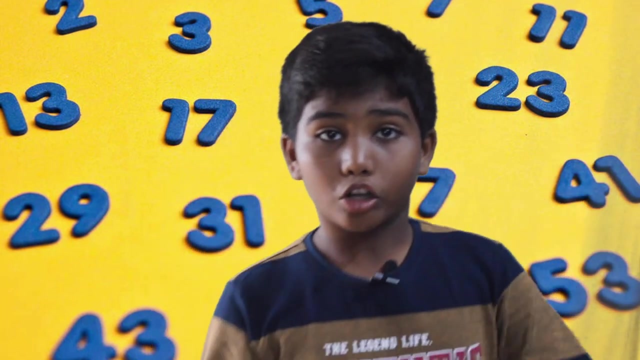 For instance, it is easy to factorize 30 as 3 into 2, into 5.. But when you are given a 7 or 8 digit number, It is not that easy to factor back that number into primes. And imagine how really hard it will be to factorize a 100 or 200 digit number. 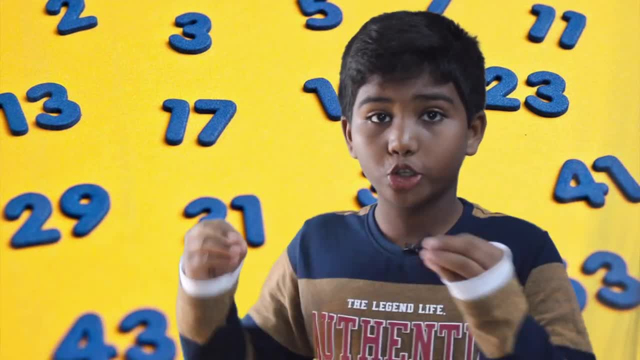 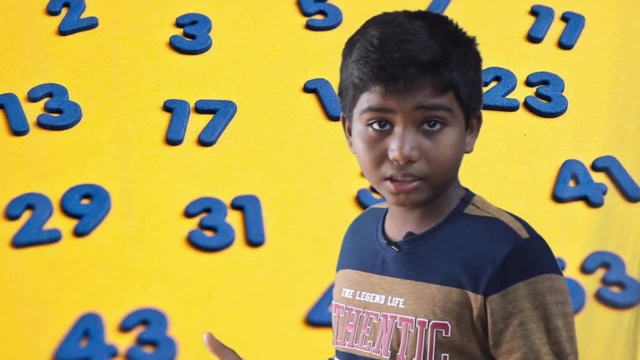 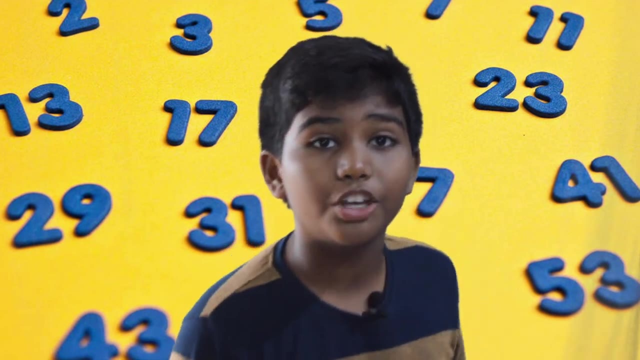 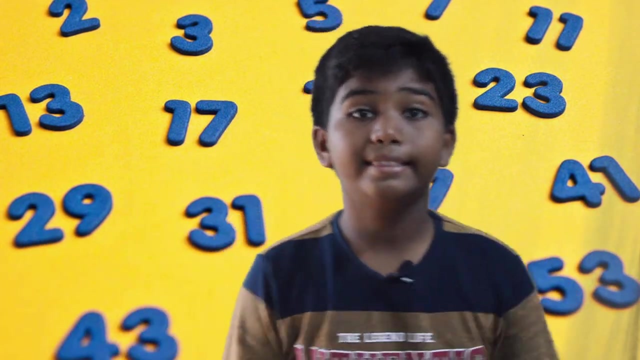 Here is where prime numbers are put to good use in encryption technology. You can pick two really large prime numbers and multiply them to get a super large number. However, if you are given a super large number, finding out which prime numbers went together to make that super large number is impossible. 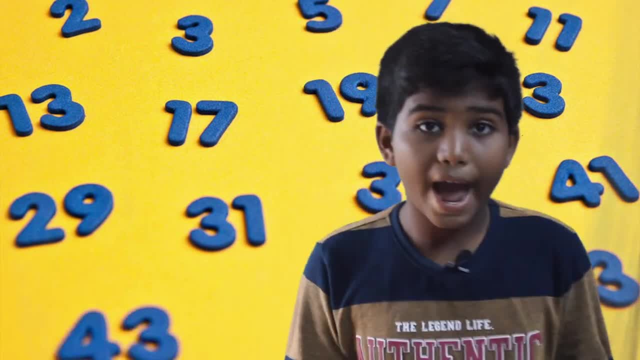 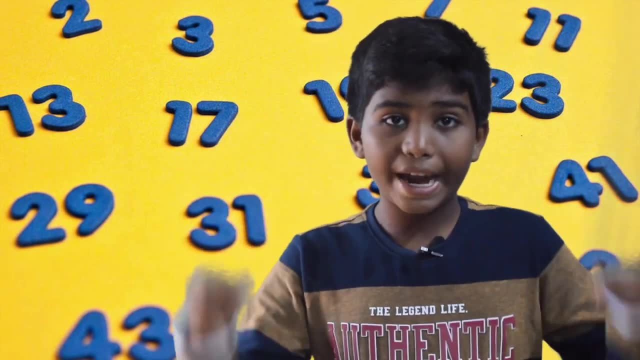 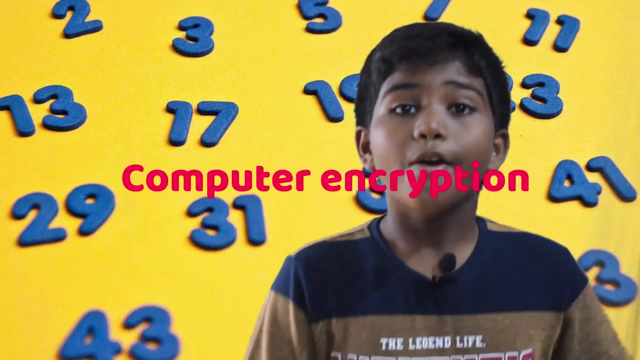 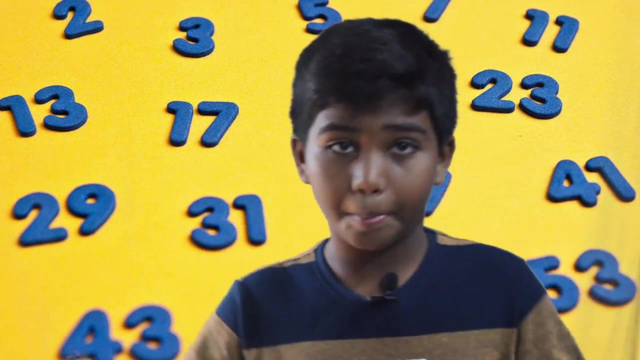 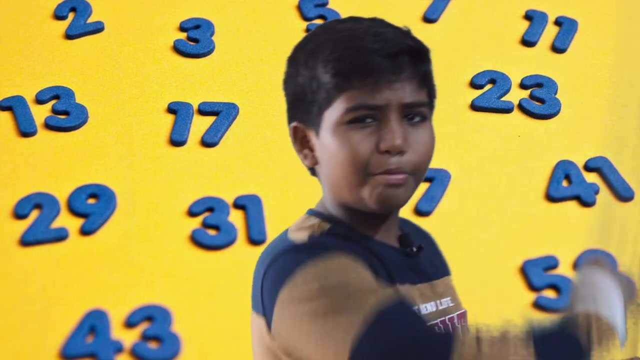 Theoretically it is not impossible, but it would take a lot of time- the amount of time that we don't have- to find those prime numbers. So in computer encryption prime numbers are used. That means Whenever you make a purchase online using your credit card or log in to your bank account or use encrypted chat or email features, you are making use of prime numbers. 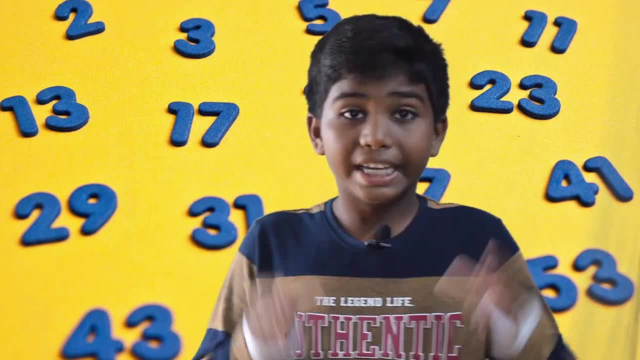 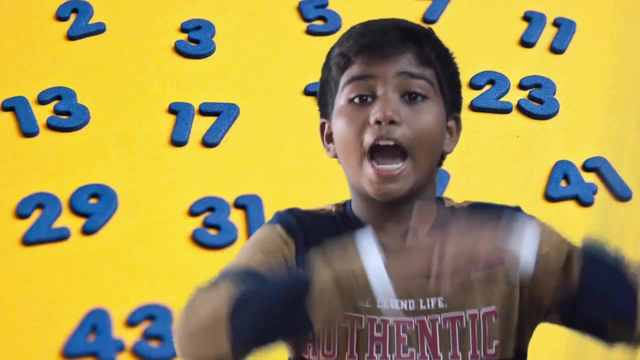 And the use of prime numbers don't stop there- In the design of turbo machinery and gas turbines for balancing reasons and for high efficiency. the number of status is not good. The number of status is not good. The number of status is not good. 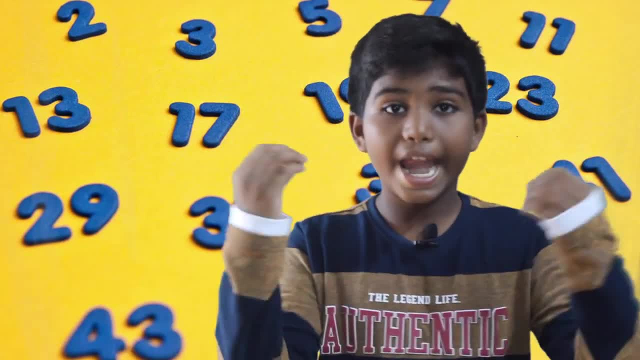 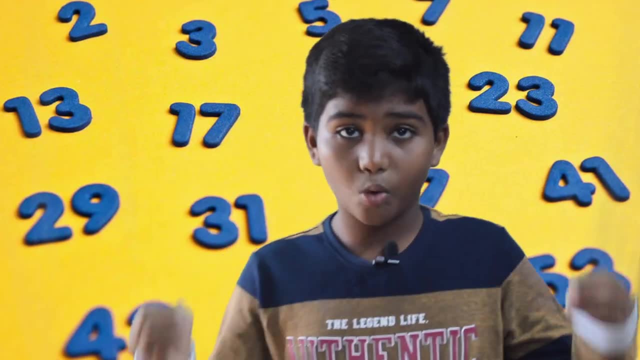 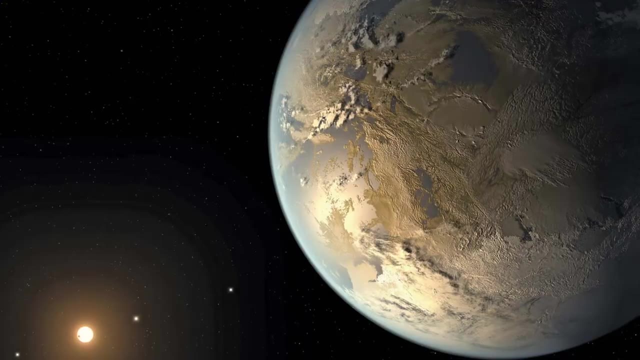 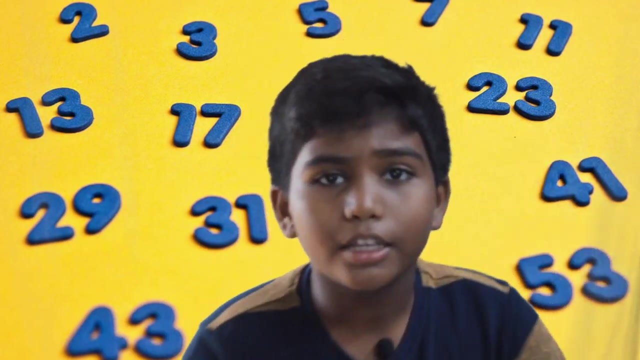 n is said to be a prime number. the enigma machine, an encryption machine used by the germans during the second world war, used primes for strong encryption. the search for extraterrestrial intelligence brings us to prime numbers too, if we ever happen to communicate with super. 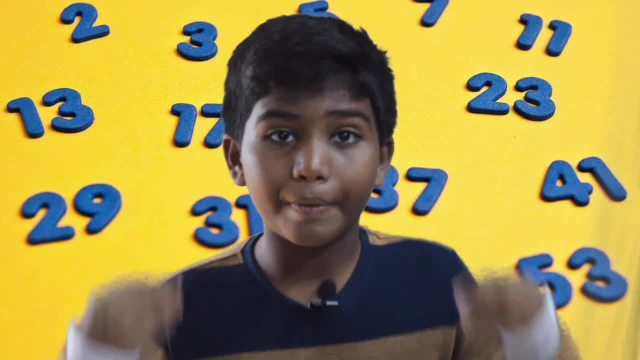 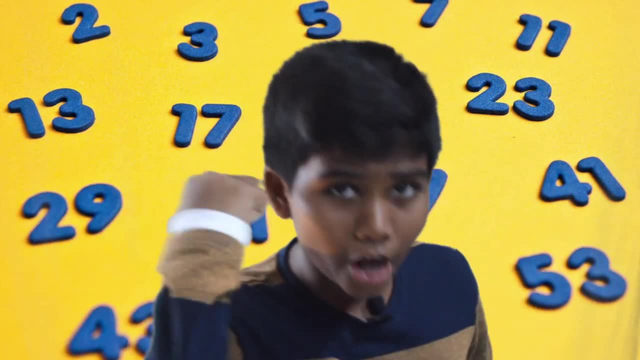 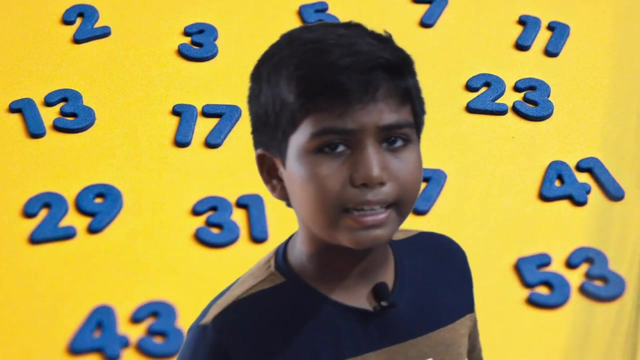 intelligent aliens, we would be using primes to send out our message. similarly, if we happen to receive a sequence of noise or a signal that is different from a normal signal in the space, and if that signal can be decrypted using primes, then it is most likely that a super 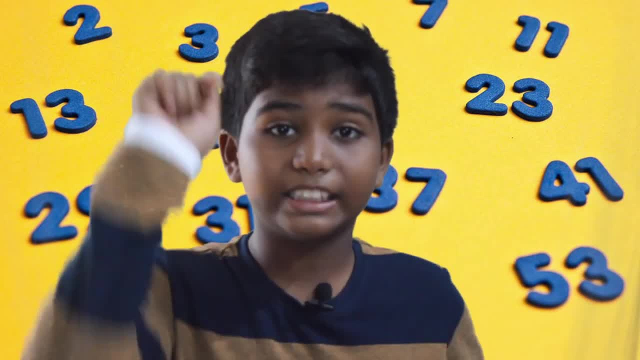 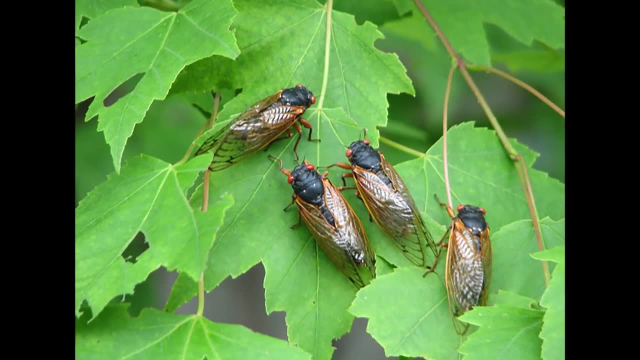 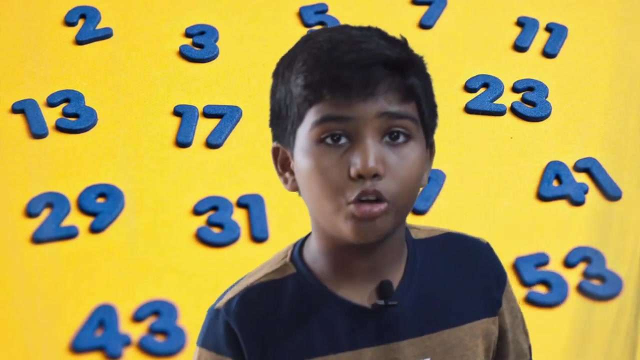 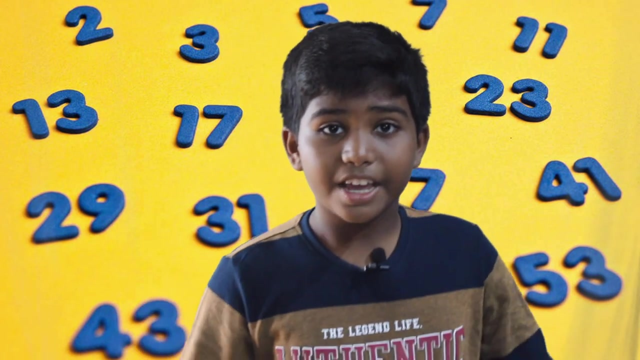 intelligent alien species exits at that space. even in the biological space, in the physical world, prime numbers are used. cicadas, a kind of bugs, hibernate for years, mostly 13 or 17 years, before they come out to breed and they die and their eggs hatch. we get to see a next generation. 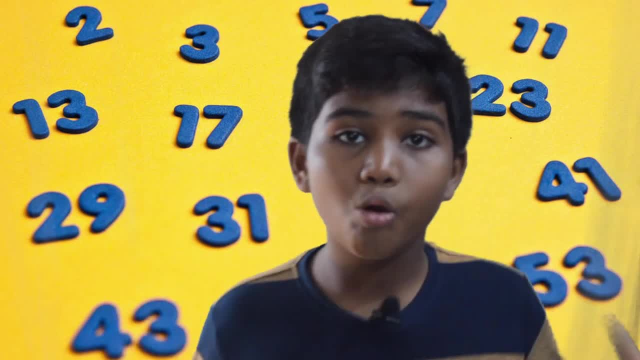 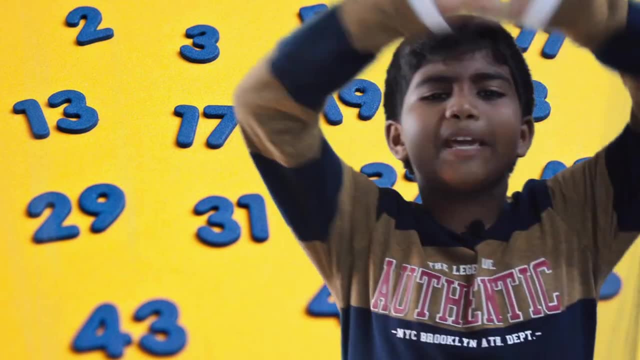 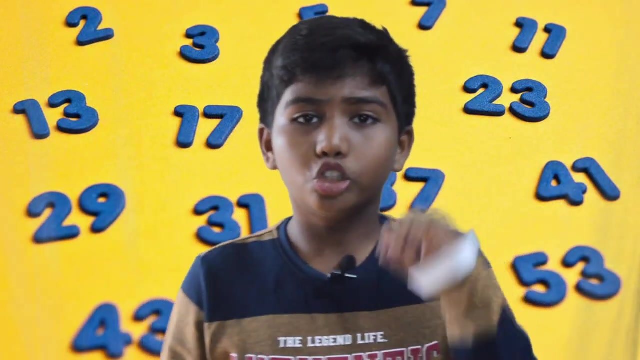 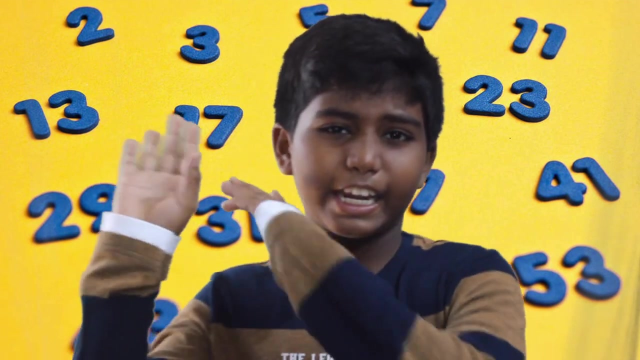 in 13 or 17 years. by spacing their outward appearance in primed years, cicadas make it least likely for any predator to jeopardize their existence. many potential predators have two to five years of life cycle, and hence that's how cicadas carry on genetically. those are some interesting uses of prime numbers.